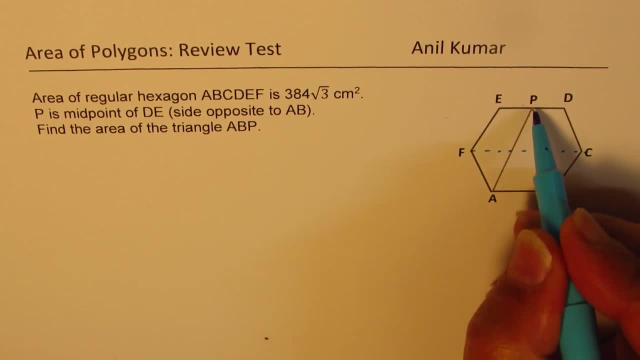 six triangles, So let's find area of each triangles. if I draw a perpendicular from here, we can actually find the area of hexagon form. we can see that this height is twice from the symmetry the height of each triangle which we can have in it right now in a hexagon. 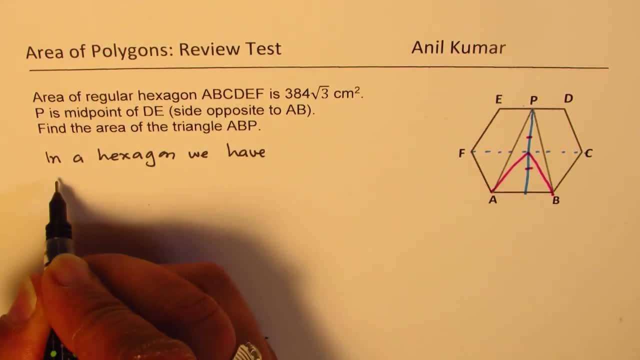 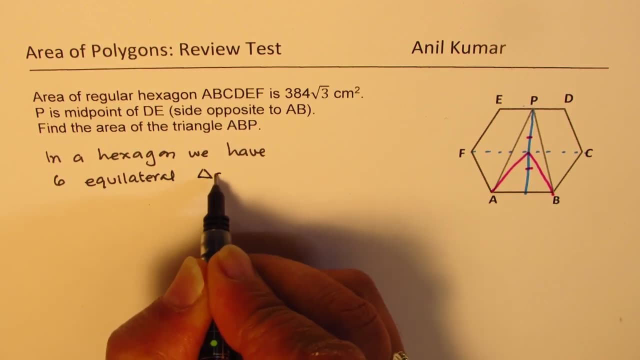 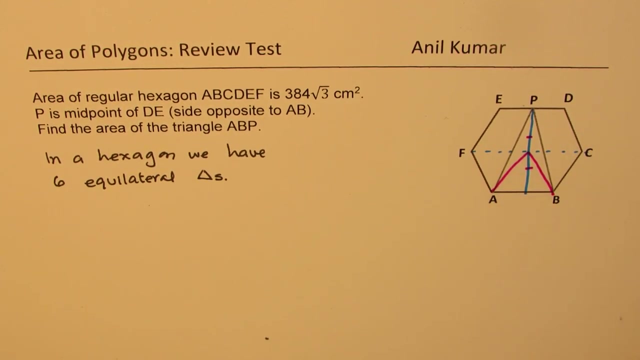 we have six equilateral triangles that, as shown, that is one of them. let us assume that this triangle which we have drawn, let me draw here, let's call this point as O. right, let's call this as Q. so in this particular triangle, let's assume that each side is 2, X. then 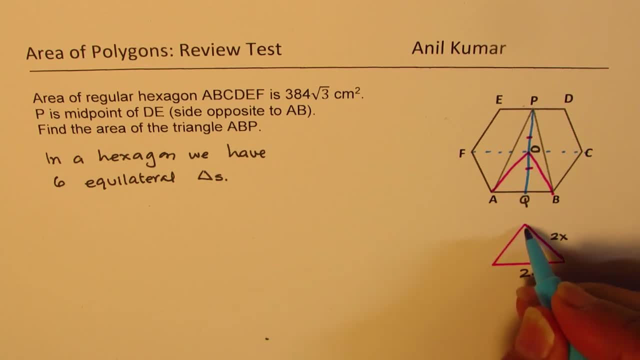 when you, then, when you, then, when you drop a perpendicular, it is going to divide this into equal parts, so this will be x and the height will be equal to what 2 x square minus x square square root, right? so this height, so in this case height, is going to be. 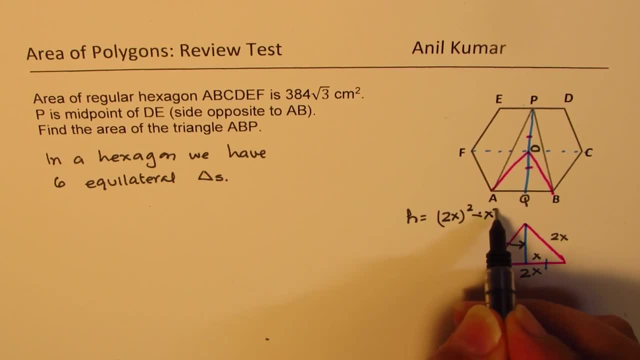 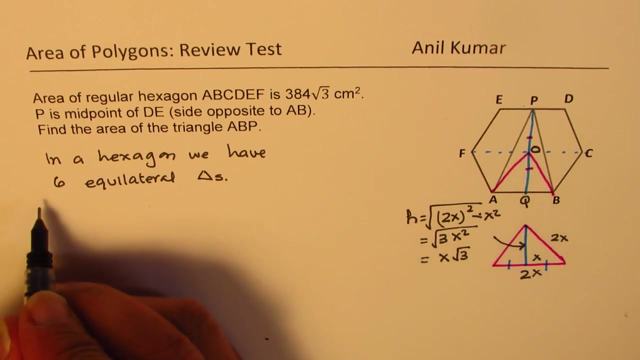 2 x whole square minus x square square root, which basically is 3 x square square root, or you can write this as x square root of 3, right? so that is the height. now, since we are given area of the whole hexagon, we can actually find area of each triangle. so 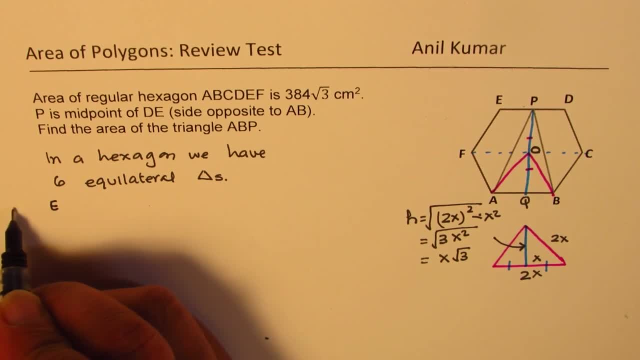 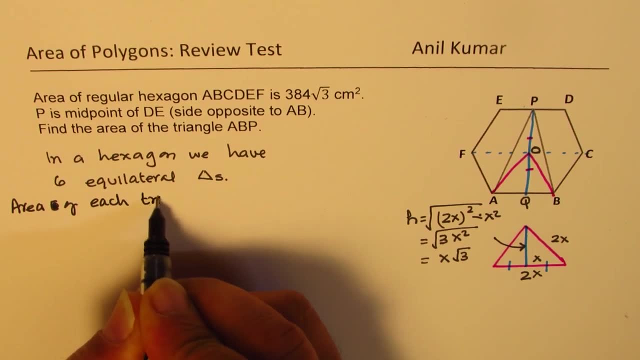 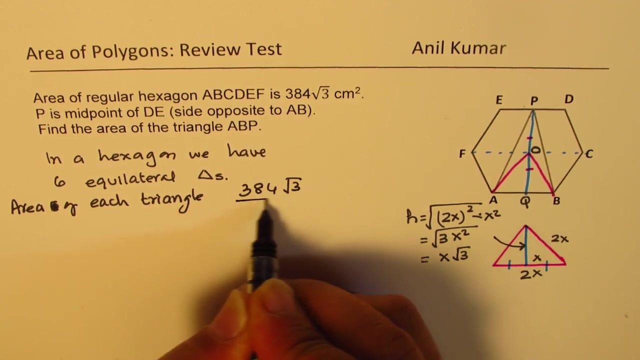 let me write area of each triangle: x square square root of x square square root of x square square root of x square square root will be given area 384 square root of 3 divided by 6. okay, so that is going to be. let's calculate. 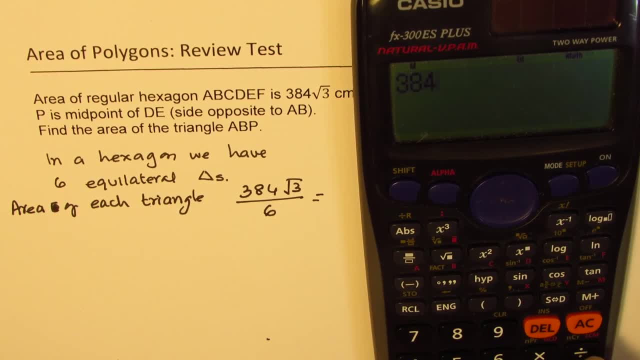 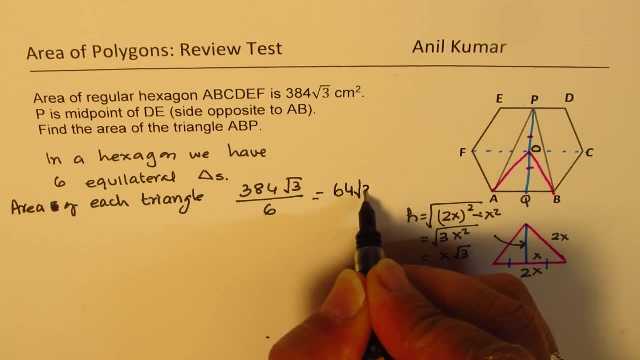 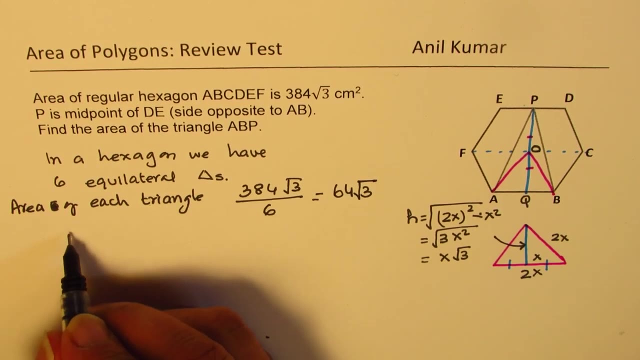 well, divide 384 by 6, we get 64 and, of course, square root 3, so we get 64 square root 3. so 64 square root 3 is area of each triangle. now we could equate this: 64 square root 3. 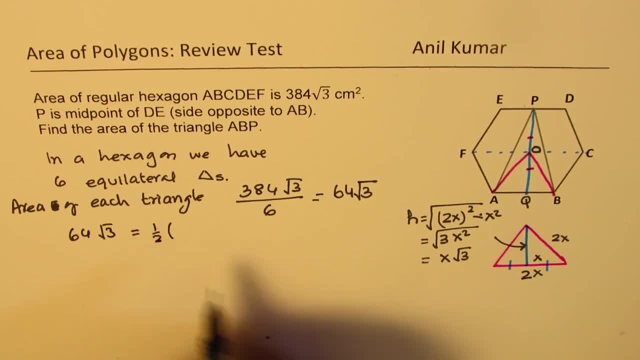 to area of a triangle which is half of base base is 2 x times height, which is x square root 3, and from here we can find side lengths. right, that's the whole idea. so if you simplify this, 2 and 2 cancel, so we get 64 square root 3 equals to x square square root 3. 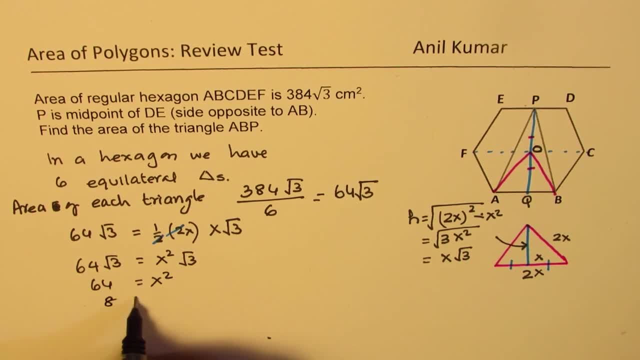 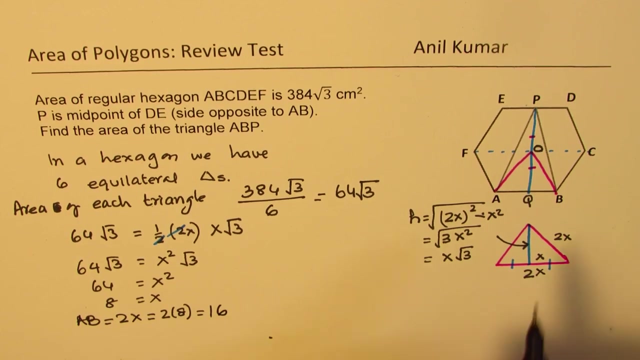 or 64 to x square, we can say: 8 is equal to x. so that means each side length is 2x, which is 16, right? so so what we get here is that the base ab, which is 2x, will be equal to 2 times 8, which is 16. so a to b, that is 16 for us. 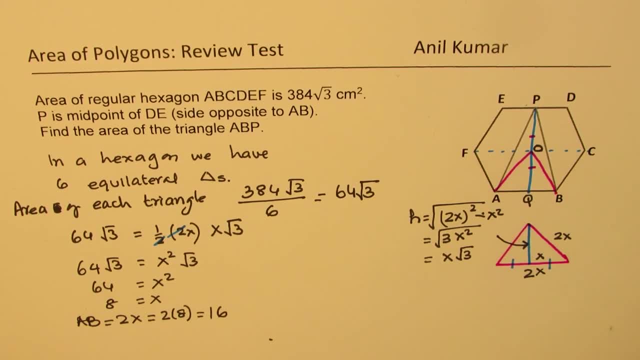 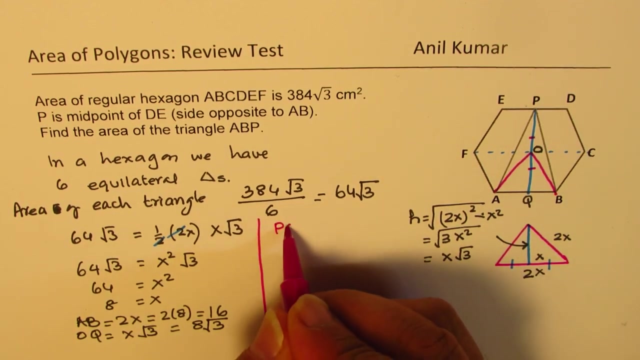 now what is oq? so let's figure this out. oq is basically x square root 3, so x is 8. so that is 8 square root 3. now pq will be how much pq will be twice oq? so that will be twice 8 square root 3, correct? 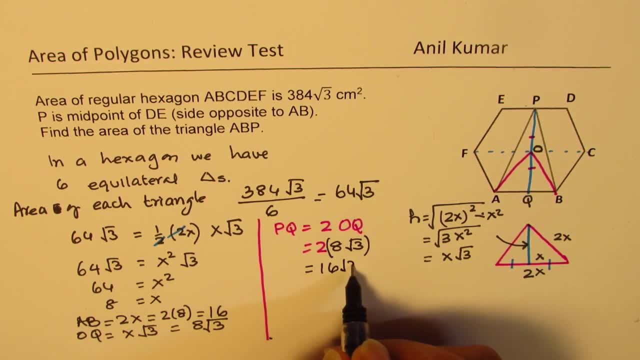 which is 16 square root 3. so for finding the area of triangle abp, we have all the required things. so area of triangle abp will be equal to half of ab, which is 16 times the total height, which is 16, which is 16 square root 3, correct. 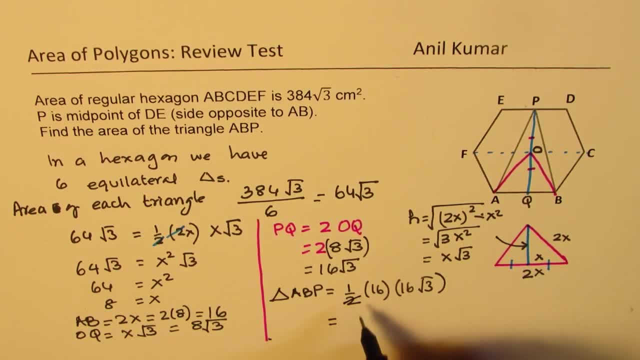 now. so we, when we calculate, we get 16 times 8 and 8 times 16, so we get 48, 8 and 4, 128 square root 3 units will be centimeter square. is that clear? so that is how we will find the area of this particular triangle.